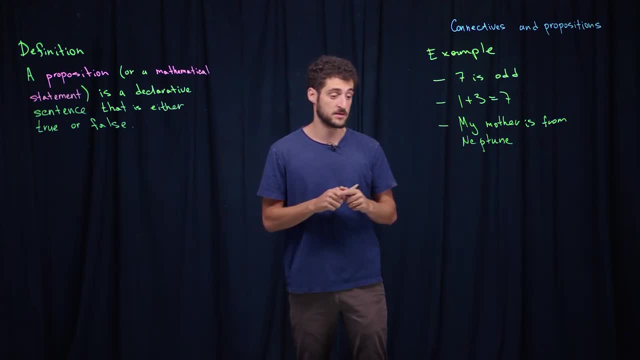 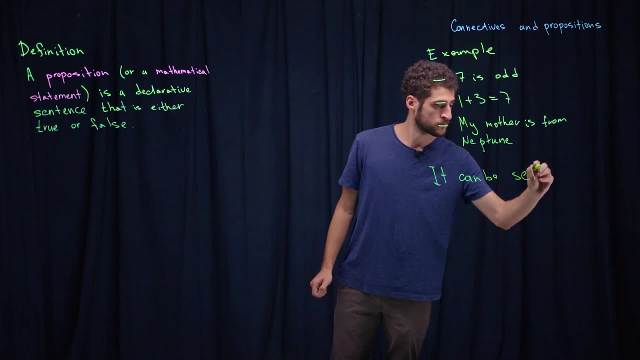 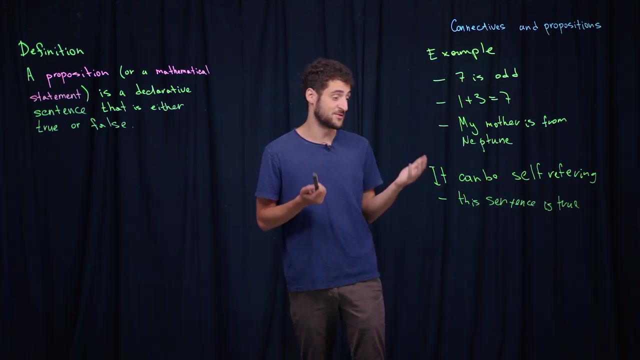 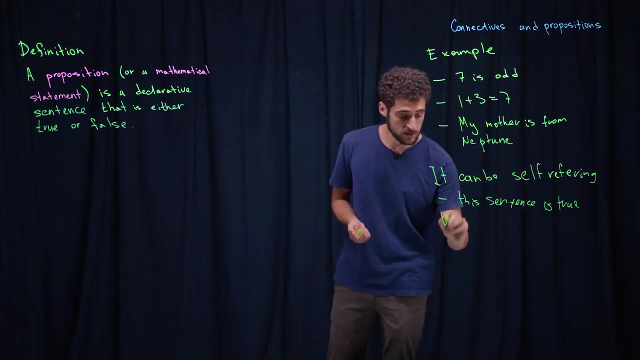 So why some sentence may not be a mathematical statement Self-referring such as: this sentence is true. We cannot determine if the sentence is true or false, because if it's true, then it's true. If it's false, then okay, it's false, Or it may use something undefined. 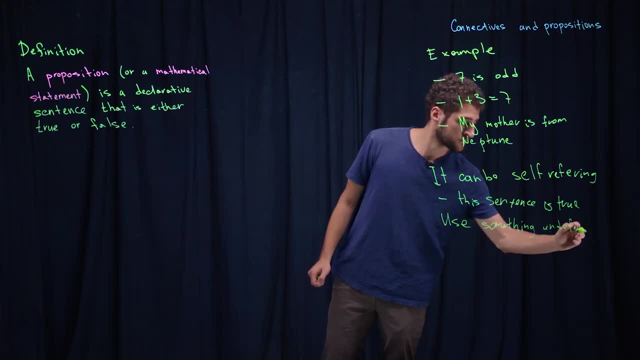 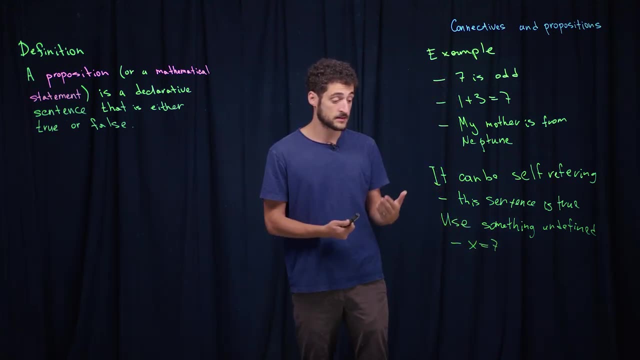 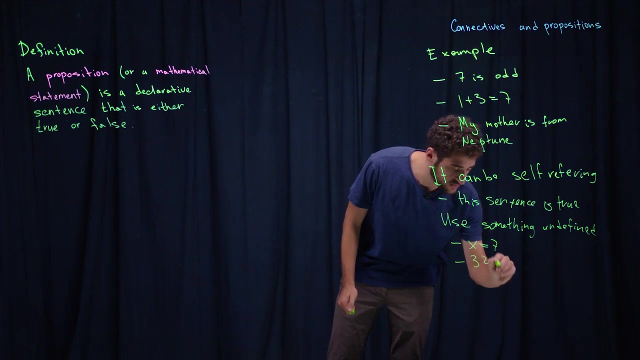 Like x is equal to 7.. Unless we define what we mean by x, we cannot check if it's true or false. So it's not a mathematical statement, Or it may be something like 32 is special. I mean again, we use the word special and we don't know what it means in mathematics. 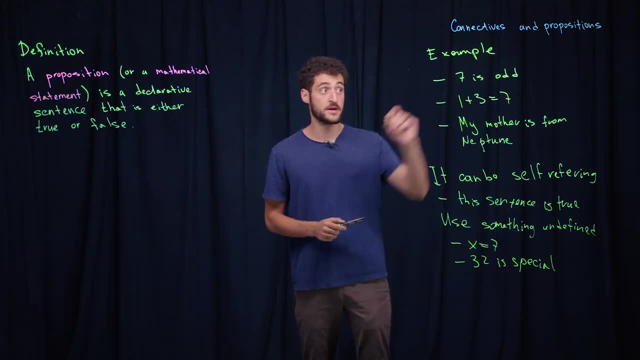 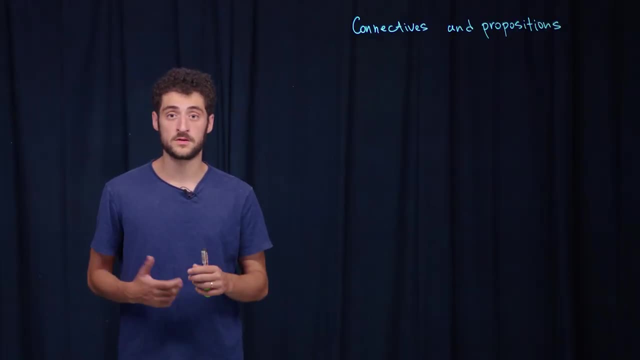 So we cannot say if it's true or false. But note that the word odd is a mathematical term, so we can use it. In everyday speech we quite often construct complicated sentences from a simpler ones. In mathematics we do the same: We use simple mathematical statements in order to construct. 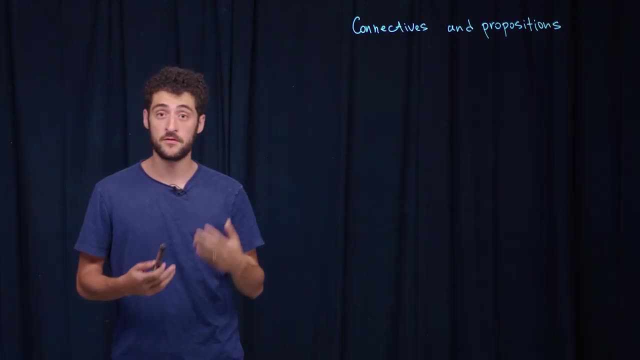 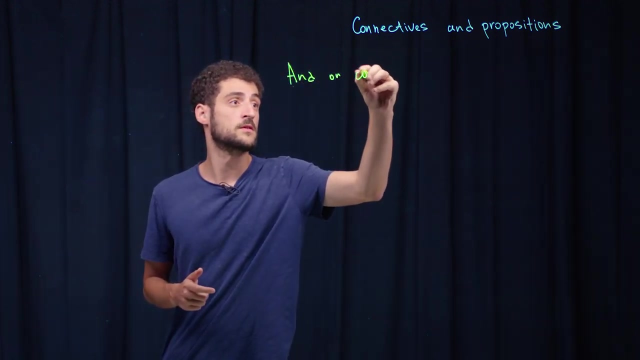 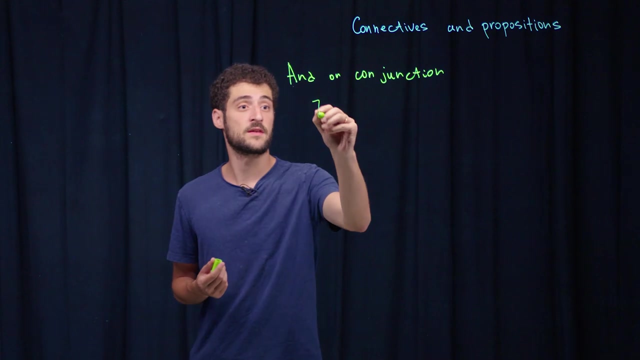 more complicated ones. In order to do this, we use connectives. The first example of such a connective is called and, or conjunction, And it's an analog of everyday speech. and For example, we may say: 7 is equal to 1 and 2 times 2 is equal to 4.. 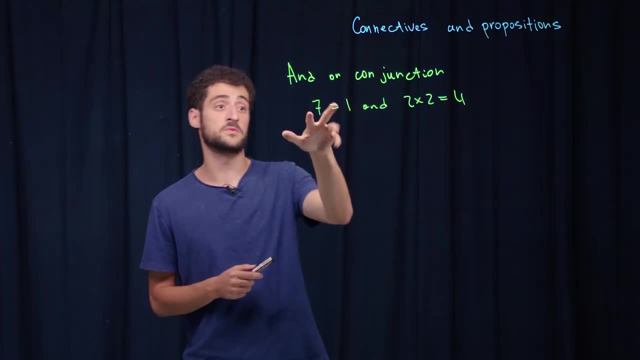 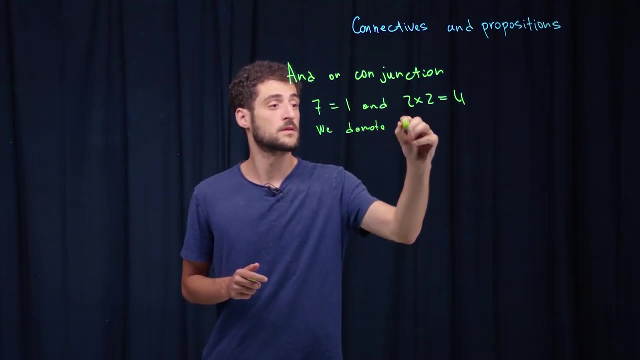 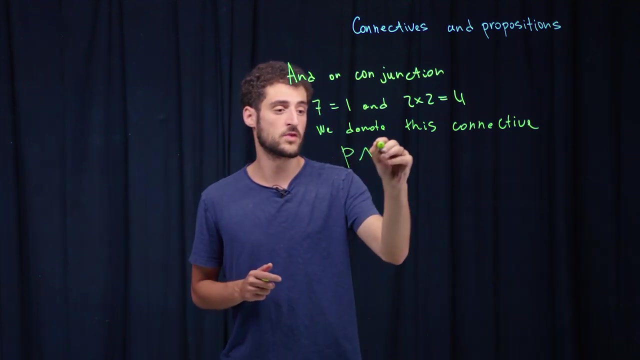 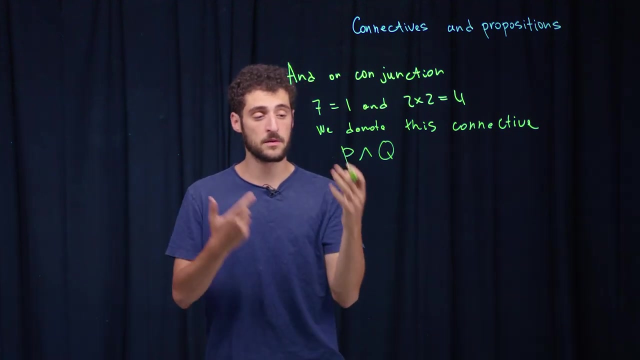 In this case it's false, because we know that 7 is not equal to 1.. We denote this connective like this, So we write p, the arrow Q, And it means that p and q And the operation can be defined in the following way: 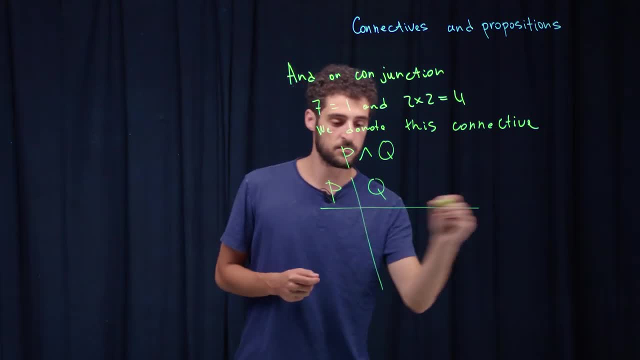 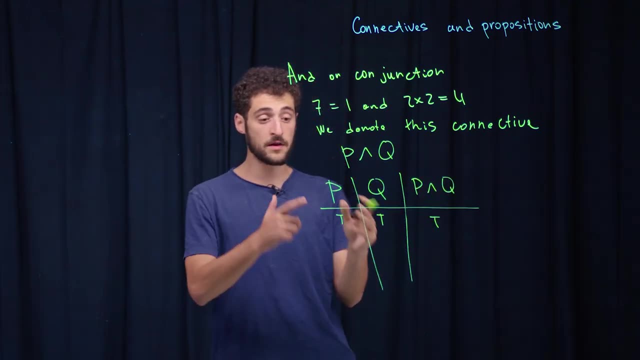 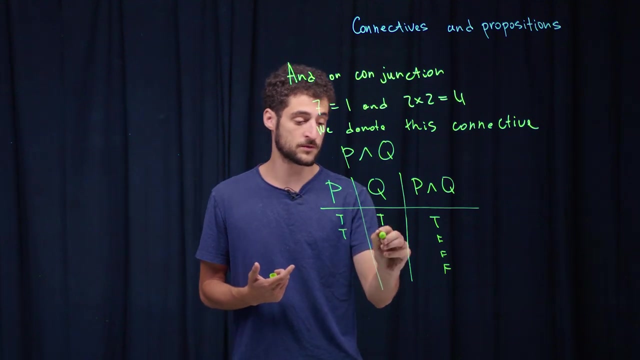 So if you know p and q, If both of them are true, Then p and q is true as well. In every other case it's false, Because if q is false, then obviously the end of these two statements is not true. If p is false, then again it's not true. 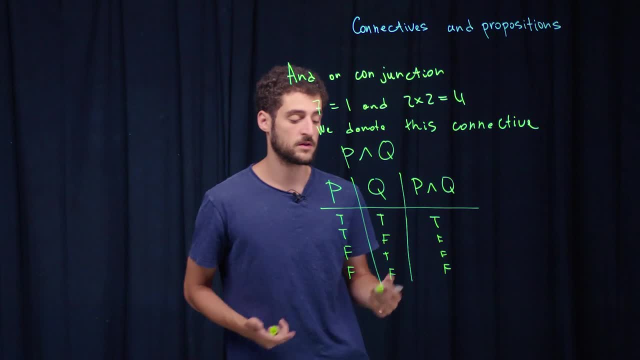 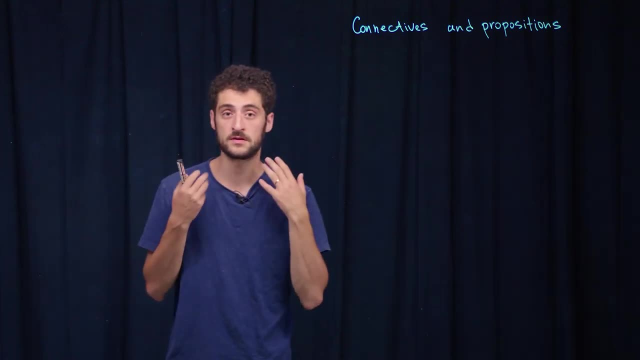 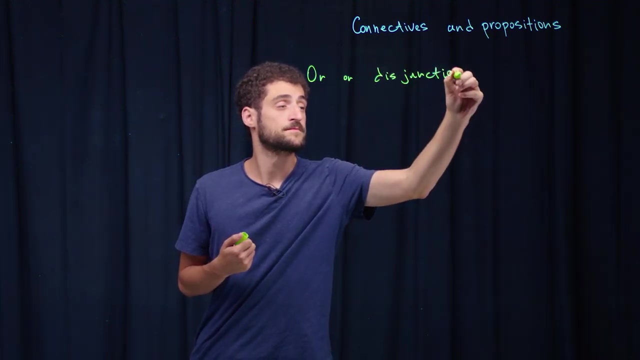 If both of them are even false, It's still a false statement. The next example of a connective is or or disjunction. So example of this connective is: 7 is equal to 1, or 2 times 2 is equal to 4.. 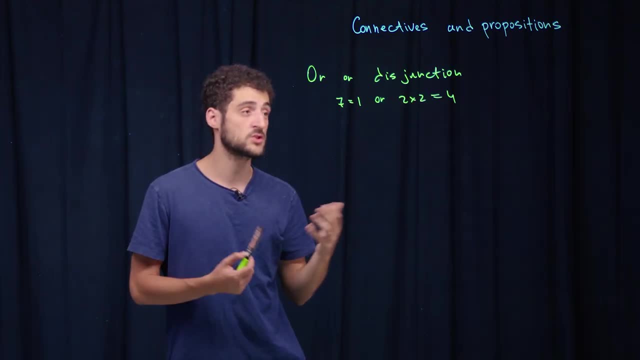 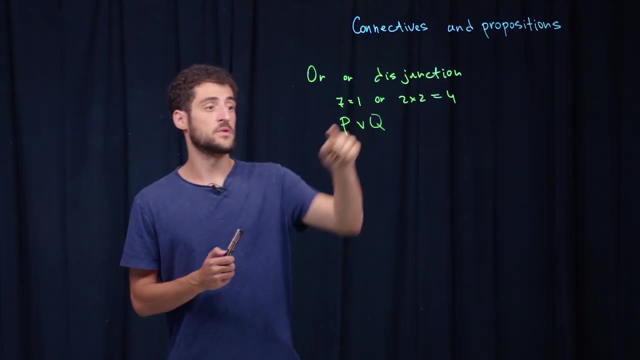 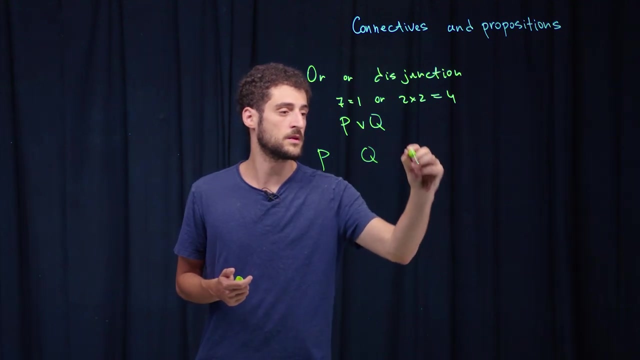 This statement is true, since 2 times 2 is actually equal to 4. And we don't care about the second part. We denote it as p or q With down sounded arrow, And the value can be determined as follows. So if you have p, q and p or q, 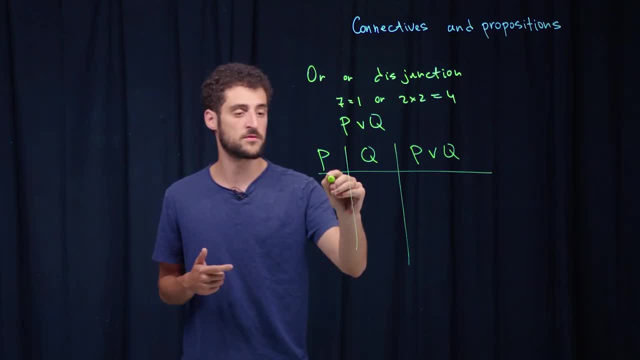 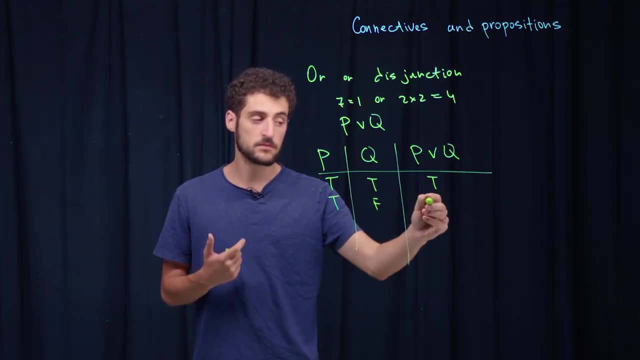 Then the truth values are the following: So if p is true and q is true, Then their or is true. If p is true and q is false, It's still a true statement. If p is false but q is true, it's also true. 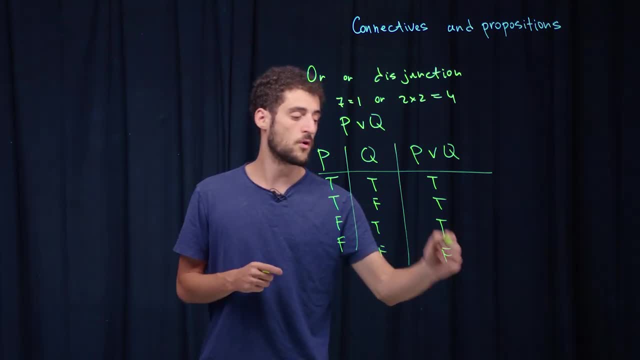 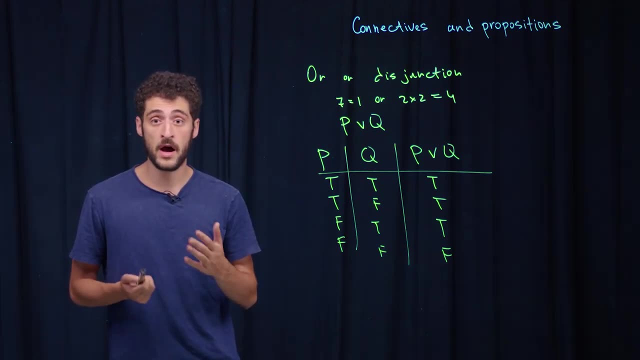 And if both of them are false, The or is false. Note that in everyday speech I may say something like I want to eat bread or caviar. It means that I don't want to eat both of them. I want to eat one of them. 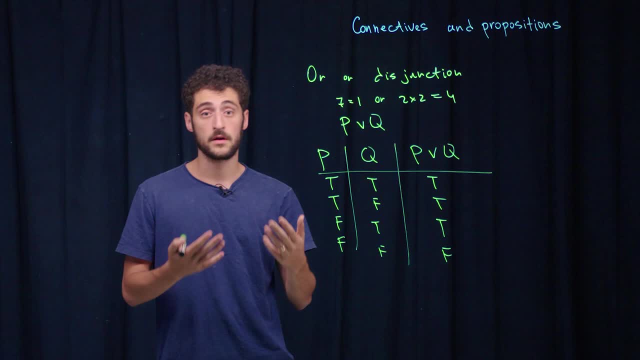 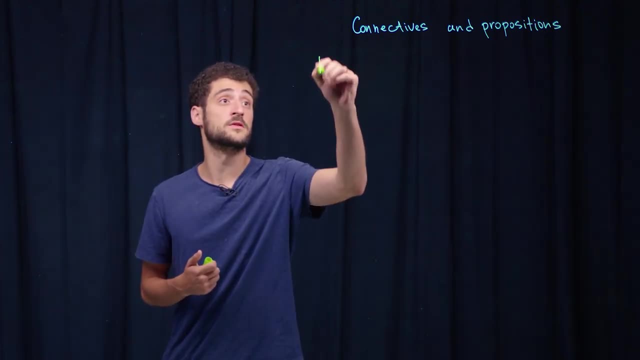 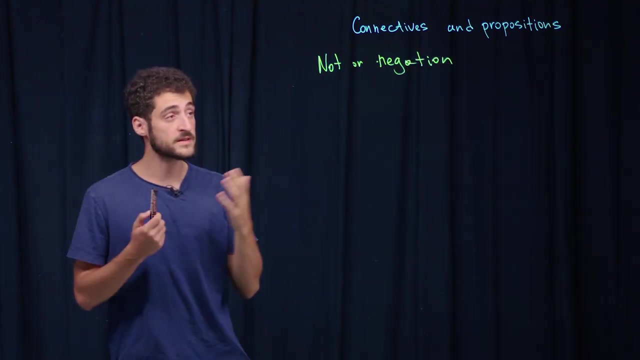 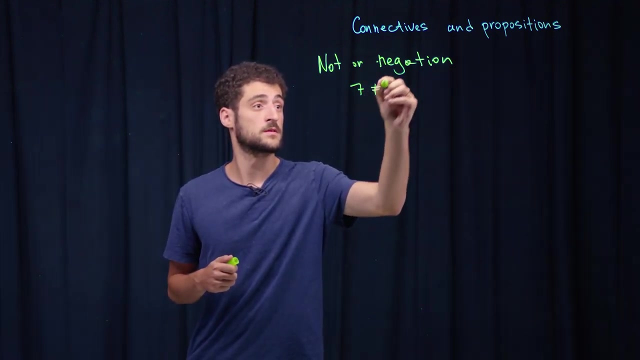 But in mathematics it's okay. if both of them are true, It's still a true statement. The last example of a connective is not, or also known as negation. So example of this may be something like: 7 is not equal to 1.. 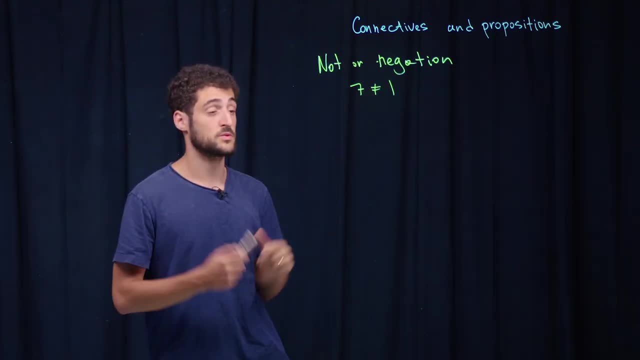 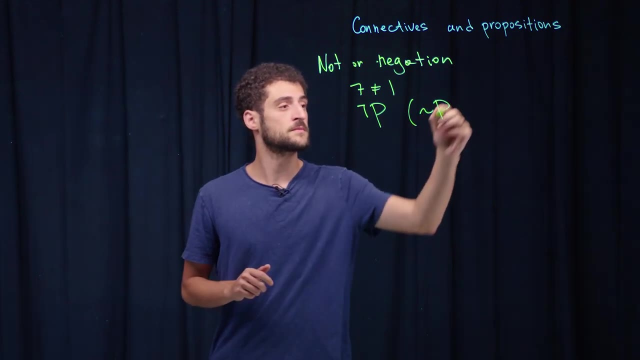 So obviously this is true, because 7 is actually not equal to 1. And we denote it as not p. Sometimes people also write it as like this, So we may define this expression like this: So if you know the truth, value of p. 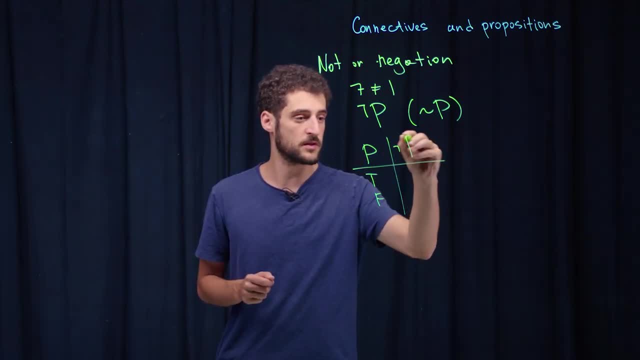 It's maybe true or false, Then the negation of p is the opposite. So if p is true, then the negation is false, And if p is false, then the negation is true. In this video we discussed propositions and connectives. 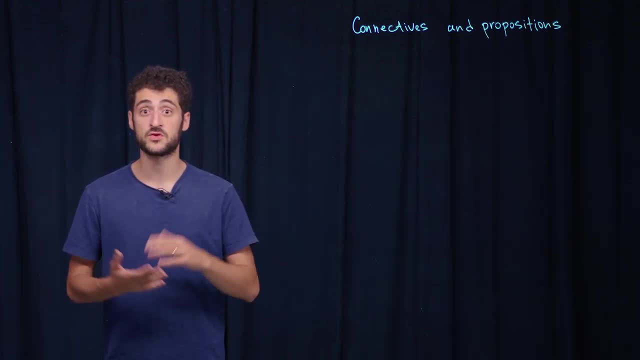 In other words, we discussed what is the mathematical statement And how to describe them. In the next video, we are going to discuss the main object in mathematics Sets.